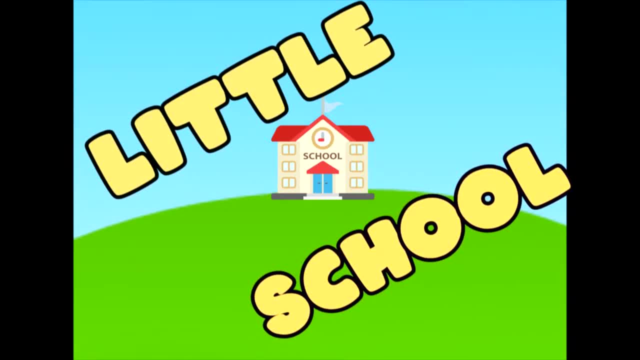 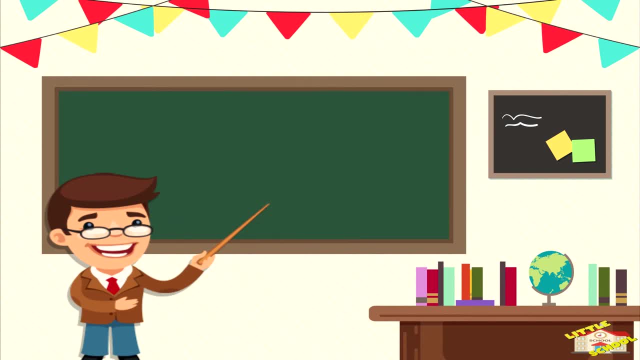 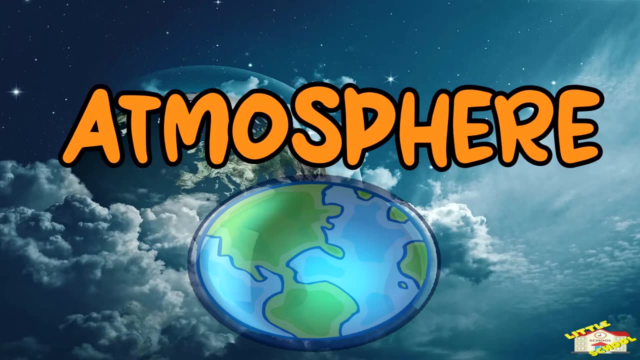 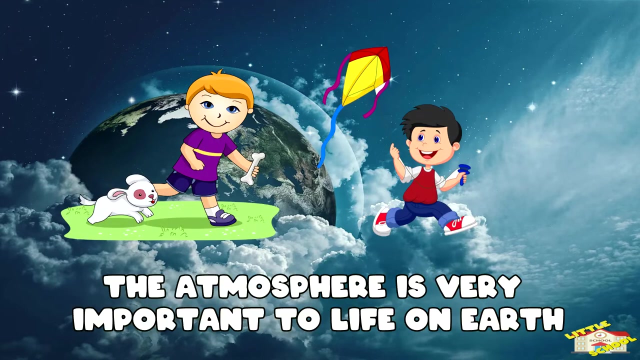 Hey kids, In today's video we'll be learning about the atmosphere. Are you ready? Let's begin. The earth is surrounded by a layer of gases called the atmosphere. The atmosphere is very important to life on earth. The atmosphere protects earth like a. 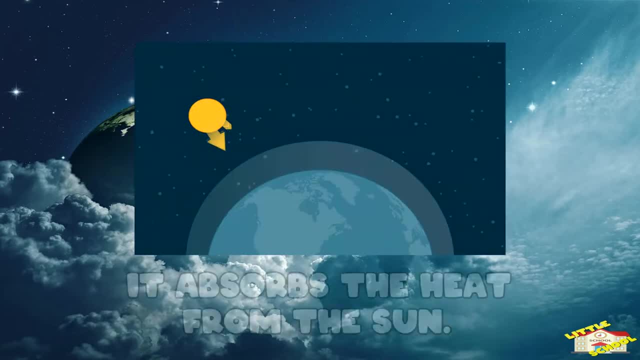 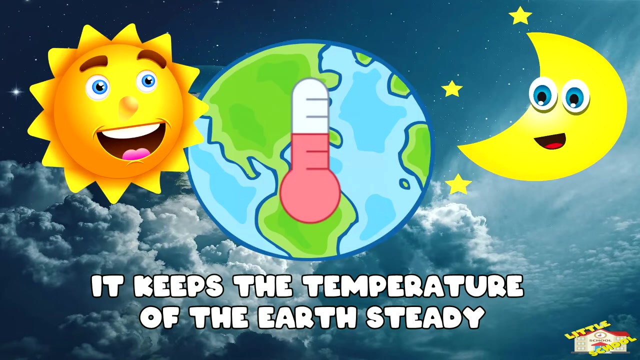 big blanket of insulation. It absorbs the heat from the sun and keeps the heat inside the atmosphere. This helps the earth to stay warm. It also keeps the overall temperature of the earth fairly steady, especially between night and day, So we don't get too cold at night and too hot. 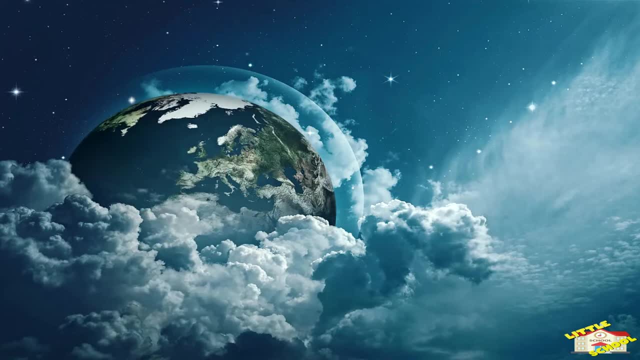 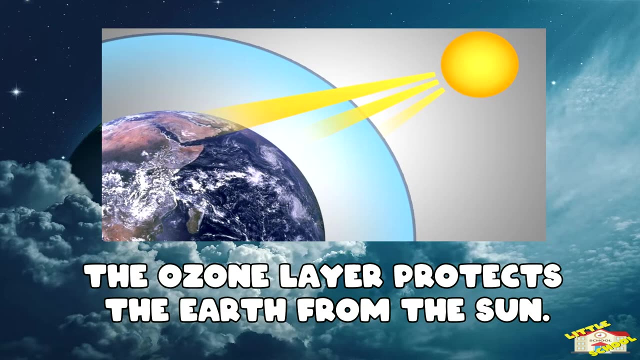 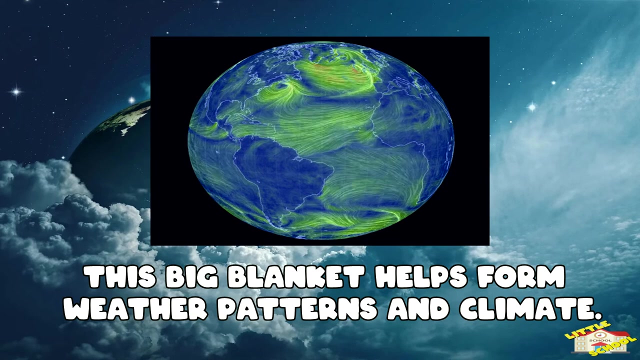 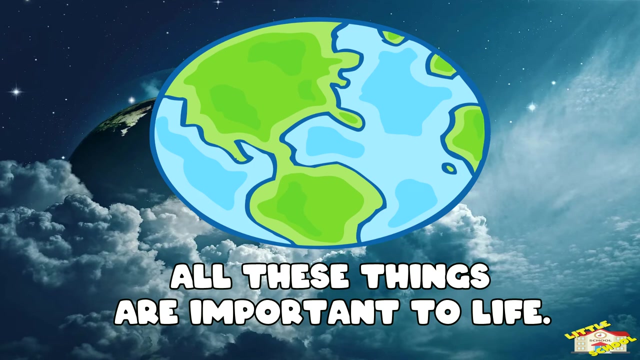 during the day. There is also a portion of the atmosphere called the ozone layer. The ozone layer helps to protect the earth from the sun's radiation. This big blanket also helps to form our weather patterns and climate. All of these things are important to life and the earth's ecology. 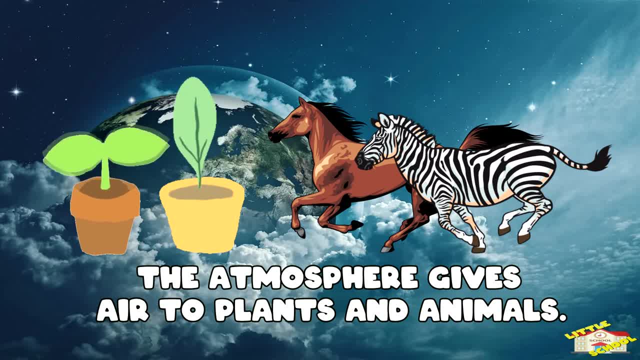 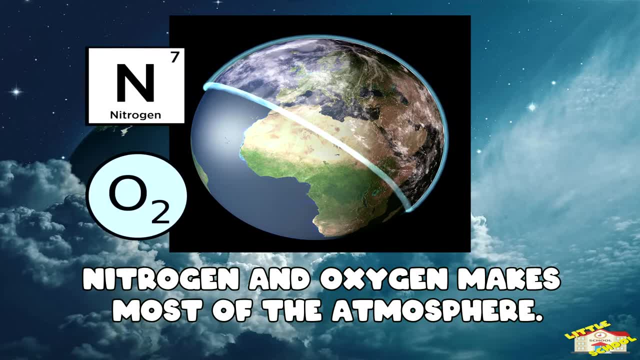 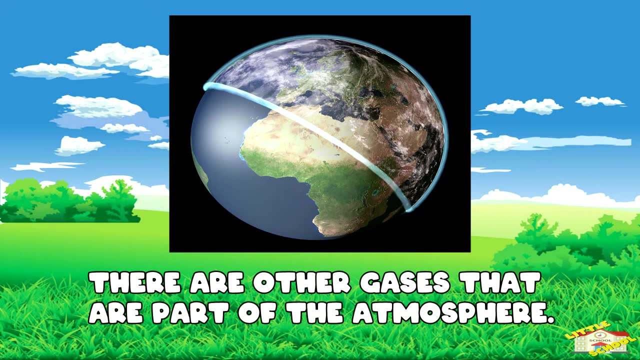 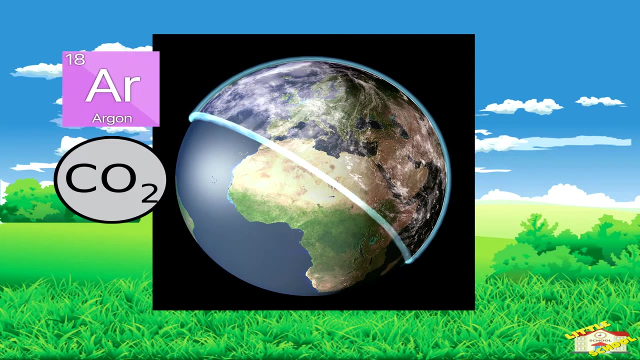 The atmosphere is the air that plants and animals breathe to survive. The atmosphere is made up of mostly nitrogen and oxygen. There are lots of other gases that are part of the atmosphere, but in much smaller amounts. These include argon, carbon dioxide, neon, helium, hydrogen and more. 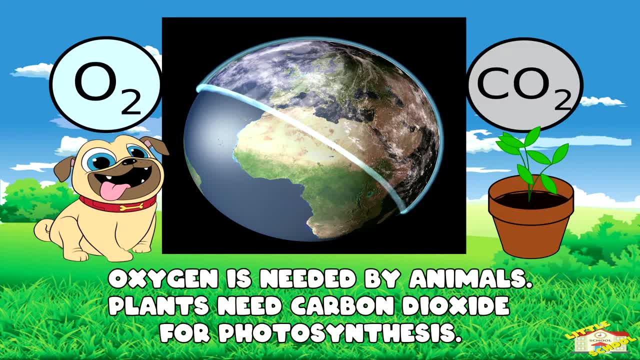 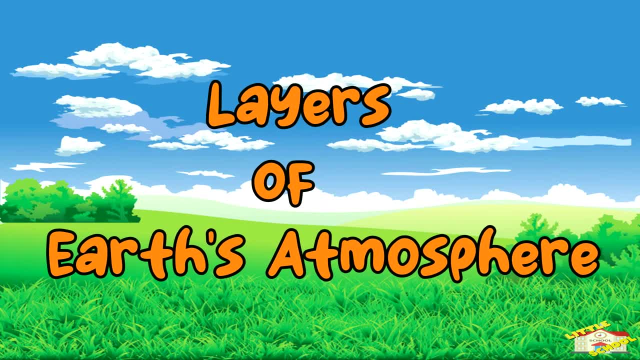 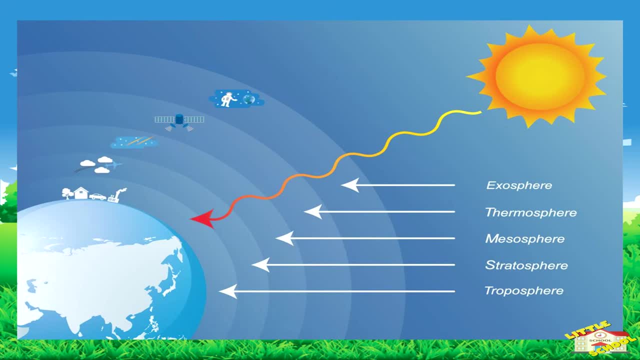 Oxygen is needed by animals to breathe and carbon dioxide is used by plants in photosynthesis. Let's go over the layers of the Earth's atmosphere. The earth's atmosphere is divided up into five major layers: The exosphere- The exosphere is the last layer and the thinnest. 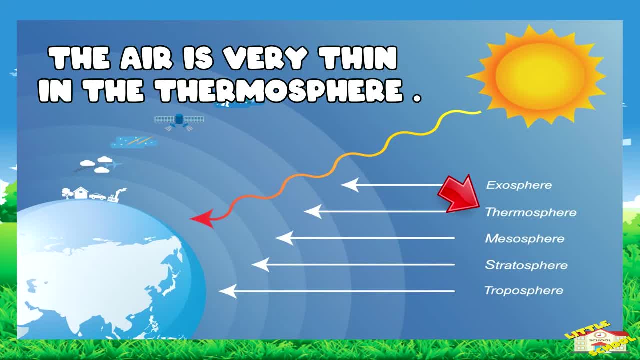 The thermosphere. The thermosphere is the next layer and the air is very thin. here Temperatures can get extremely hot, The air's marking the highest level and temperature can get much higher. Many of these really get garage air tinctures grained into cooperation with solar panel air. So all these things are important in individuals. Let's go over the layers of earth's atmosphere. 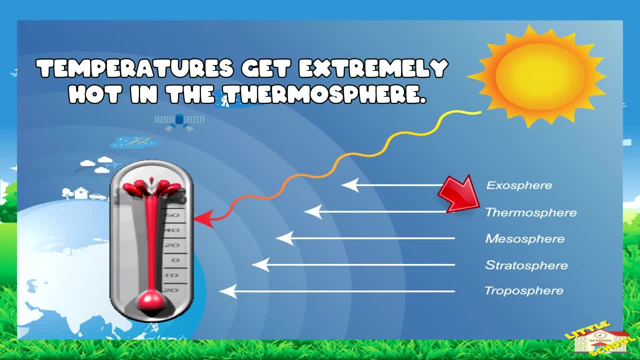 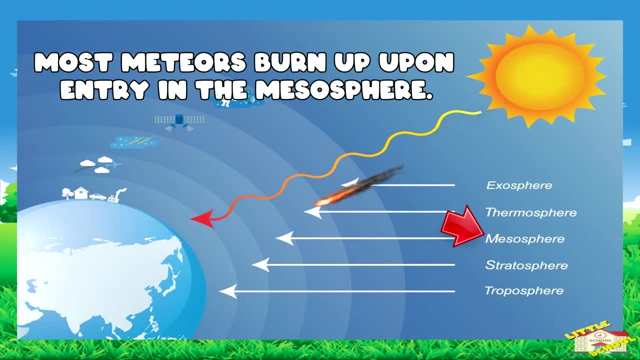 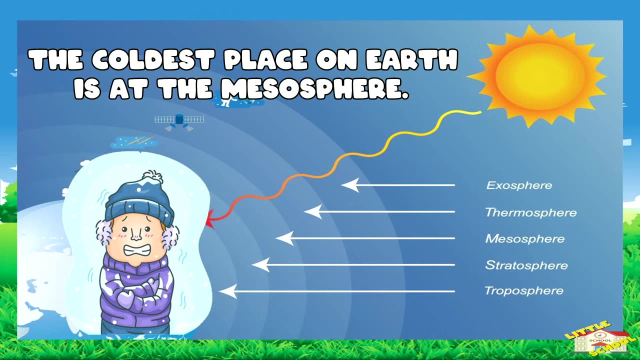 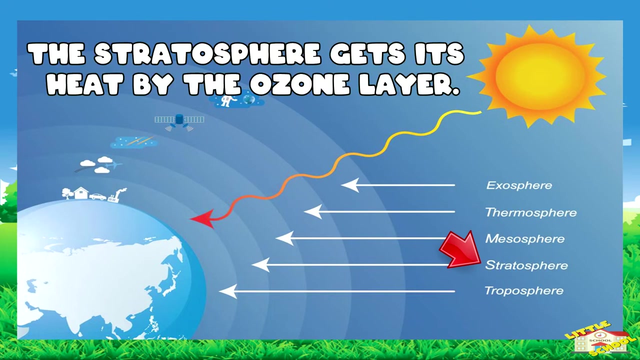 get extremely hot in the thermosphere, The Mesosphere. This is where most meteors burn up upon entry. The coldest place on Earth is at the top of the mesosphere, The Stratosphere. Unlike the troposphere, the stratosphere gets its heat by the ozone layer absorbing radiation. 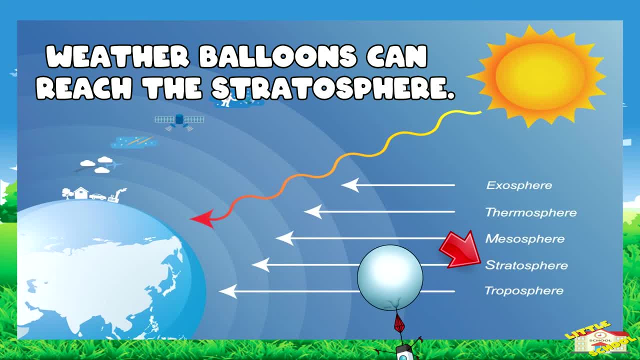 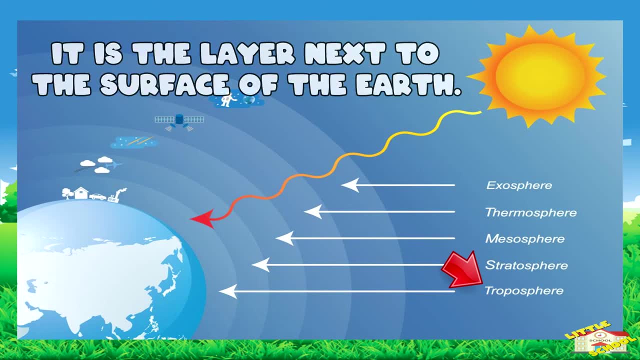 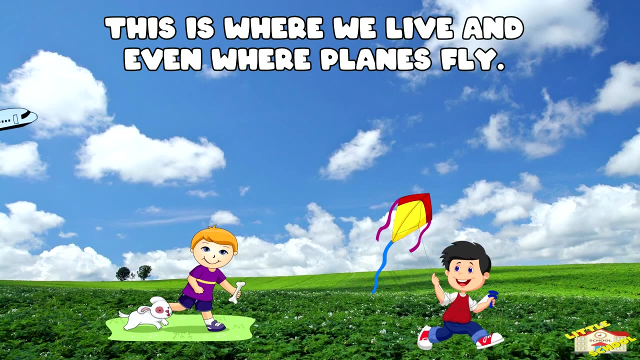 from the sun. Weather balloons go as high as the stratosphere. The Troposphere- The troposphere is the layer next to the ground or surface of the Earth. It covers around 30,000 to 50,000 feet high. This is where we live and even where planes fly. 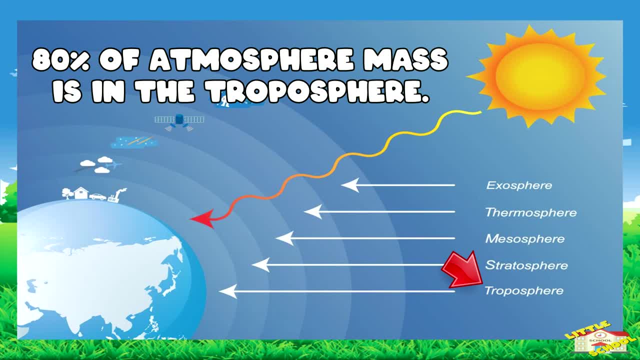 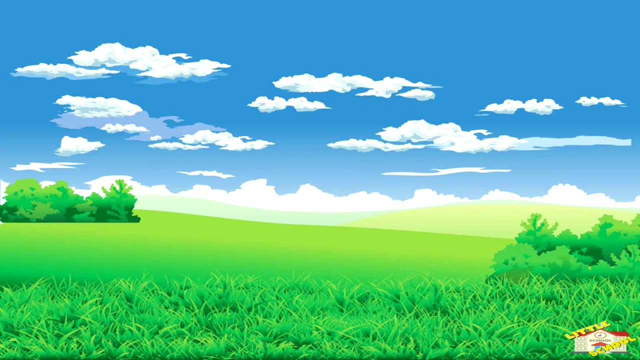 Around 80% of the Earth's surface is covered by the stratosphere. The mass of the atmosphere is in the Trophosphere. The Trophosphere is heated by the surface of the Earth. Here are fun facts about the Atmosphere. It is thought that the atmosphere that surrounds the Earth has been there since its formation. 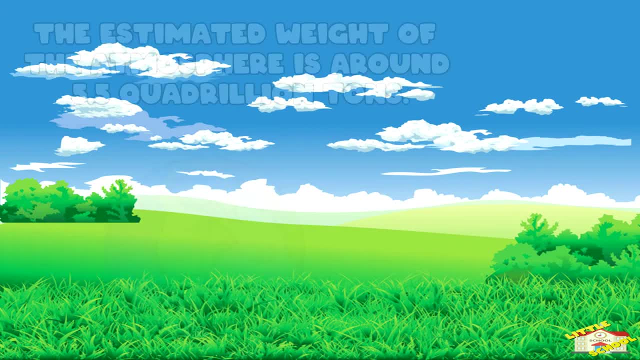 4.5 billion years ago. Earth's atmosphere is estimated to weight around 5.5 quadrillion tons. Since its formation of the atmosphere 4.5 billion years ago, Earth's atmosphere has been around the Earth for nearly 20,000 years. 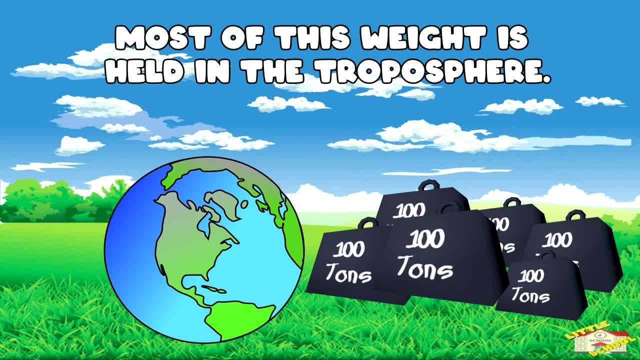 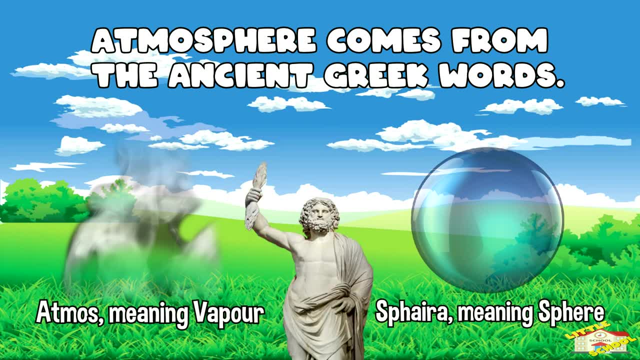 This atmosphere is estimated to be 4.5 quadrillion tons. Most of this weight is held in the troposphere, which is the level closest to Earth. The name atmosphere comes from the ancient Greek words atmos, meaning vapor, and spira, meaning spear. 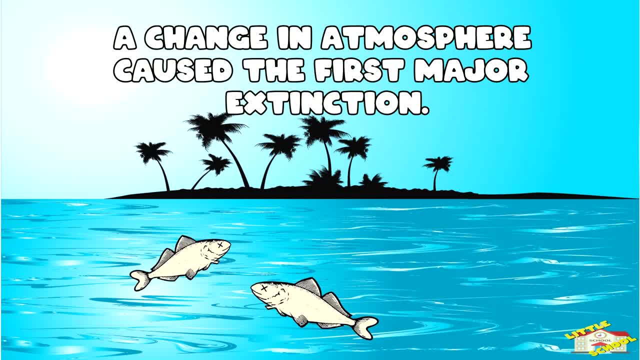 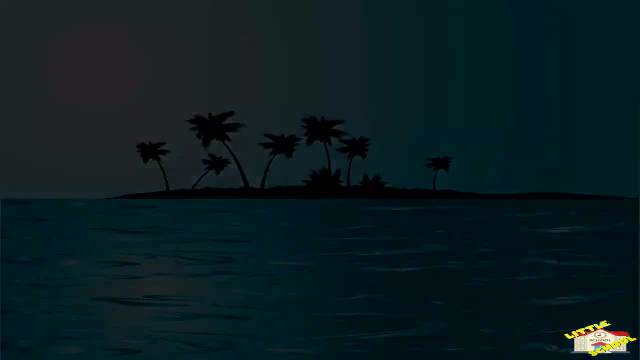 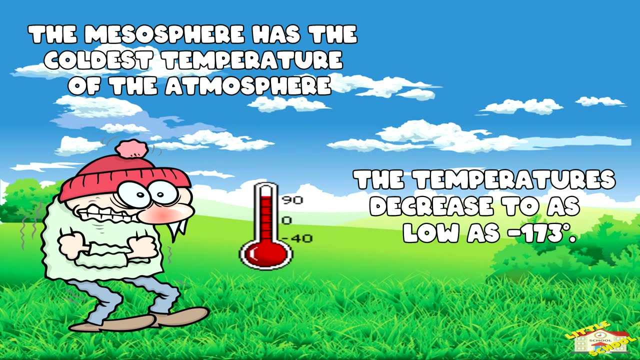 420 million years ago, the change in atmosphere caused the first major extinction, which wiped out 23% of all marine animals. The mesosphere has the coldest temperature of the atmosphere that surrounds our entire planet, where the temperature decreases to as low as negative 173 degrees.